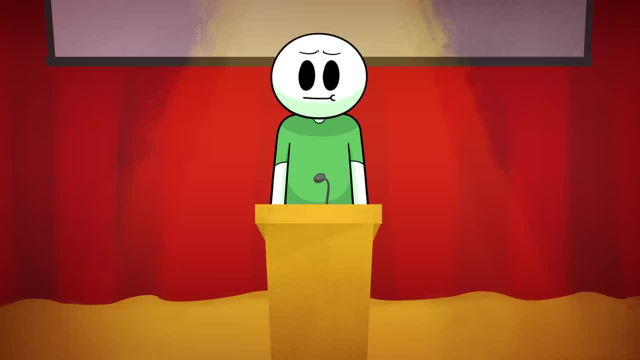 Public speaking is one of the most common fears, so you may find that shocking, And if you are like most people, you have only one question on your mind. Now that I have a violent stranglehold on your attention, I can tell you about the best presentation that I have ever given. 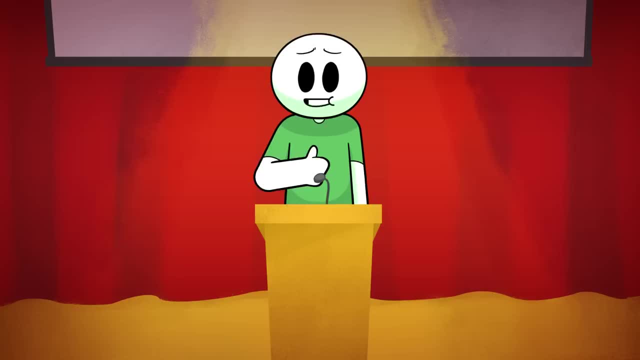 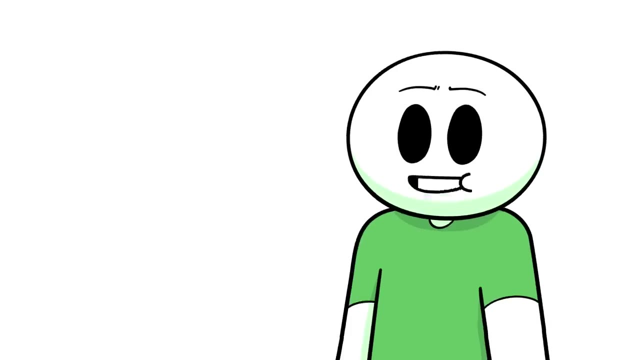 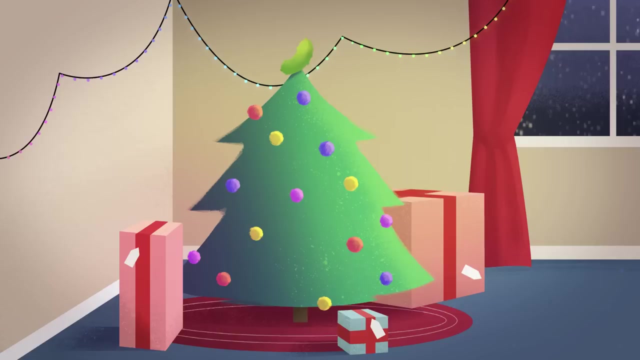 And let you in on my secret for how to be as good at them as me. One time in English class we had to give a presentation about our family traditions and trace them back to the countries they started in, Like how some parents hide a pickle-shaped ornament on their Christmas tree and give an extra present to the first kid who finds it on Christmas morning. 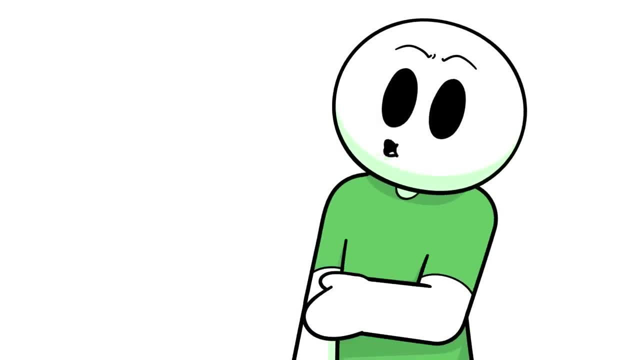 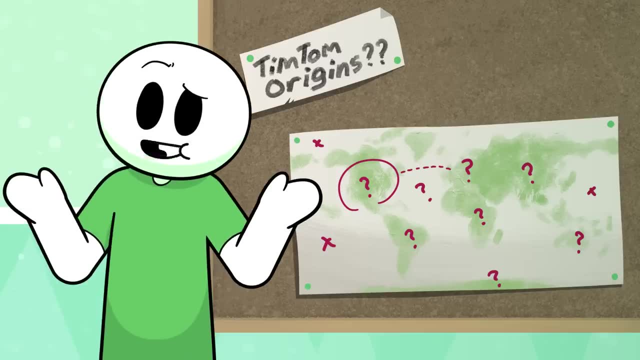 That tradition supposedly originated in Germany, but I'm not totally sure because I'm not German. Probably My mom didn't know what countries our ancestors were from. so instead of calling up distant relatives and doing, you know, research, I went to my teacher and was basically like: 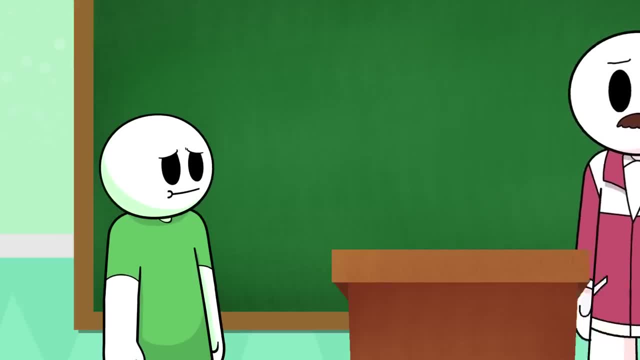 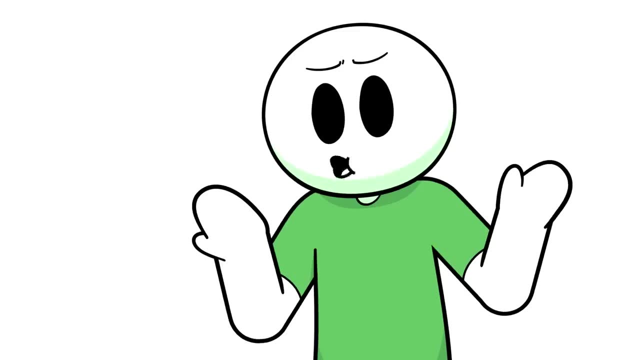 I don't have a dad, Which probably made him super uncomfortable, so he decided not to make me do that part of the assignment. For those of you keeping track at home, my assignment had just become Talk about your family, Which doesn't require any research Score. So for like two weeks the whole class would spend English class and I would have to do a whole class of English. So for like two weeks the whole class would spend English class and I would have to do a whole class of English class. 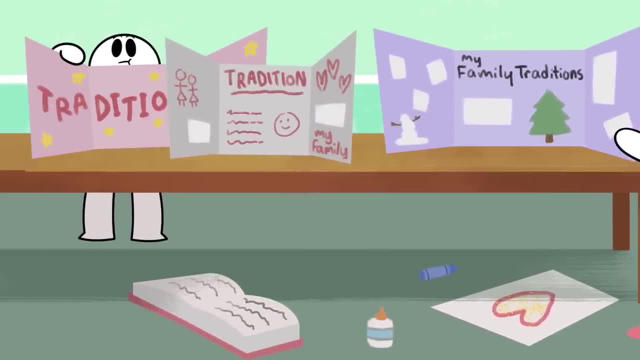 So for like two weeks the whole class would spend English class and I would have to do a whole class of English class would spend English period in the library doing research and making poster boards for their presentations- Except for me, I played computer games and it seemed like the fun would never end. 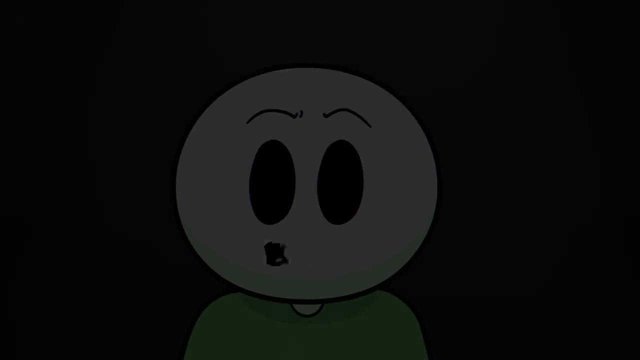 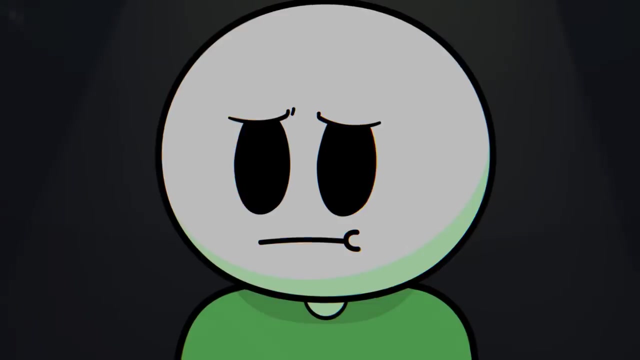 Until it did Uh-oh. Back to the scary part. Okay, I don't have anything done yet And presentations start today. What did I even do all week? We won't get through every one in one day, right? If I don't get called on, that gives me an extra day to get ready. 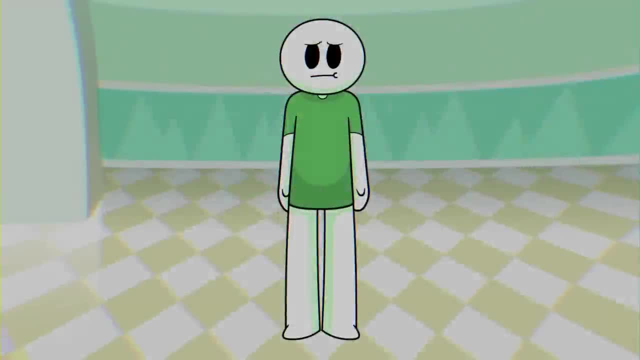 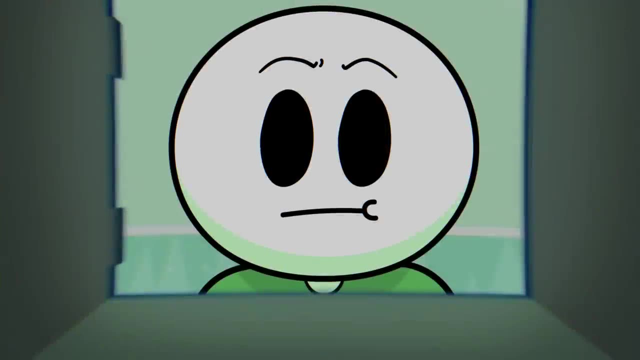 But I'll work through lunch so I'm not totally empty-handed, just in case. Yeah, that's not happening. Maybe if I don't move- move he'll forget I exist. I can't believe that worked. I can do my math homework during. 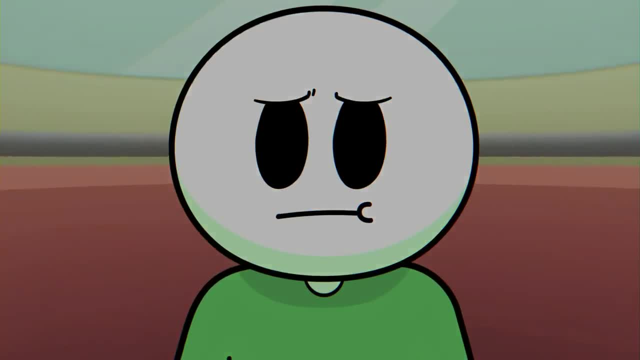 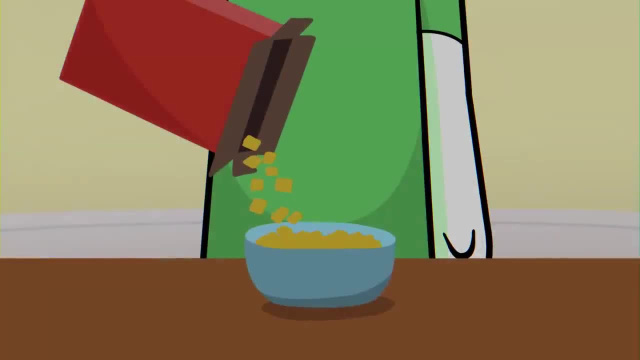 Spanish tomorrow, so the presentation is the only thing I have to worry about tonight. Oh, I'm way too stressed to get anything done right now. I just need to relax for a second. Why can't I think of what to write? I thought this was going to be really easy. 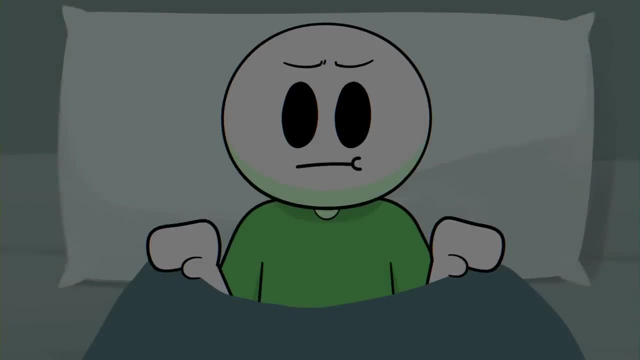 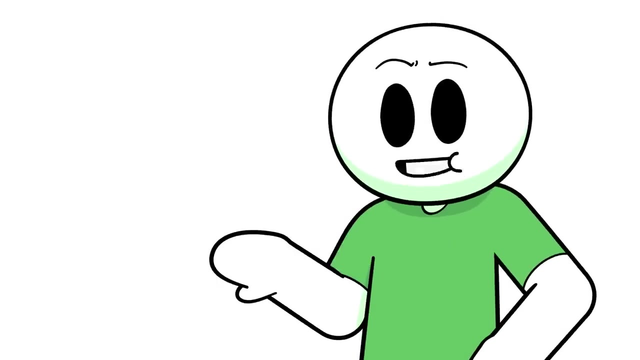 but I've got nothing. Well, let's just hope I don't get called tomorrow. I've got it. I wake up in the night with ideas all the time. Usually it's dumb ideas for videos, but I'm too tired to know how dumb they really are. so the next morning I find things like: 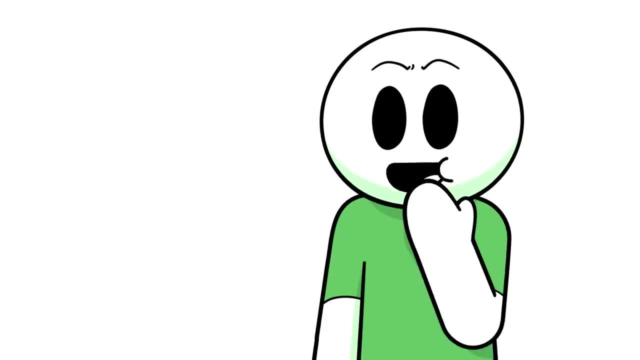 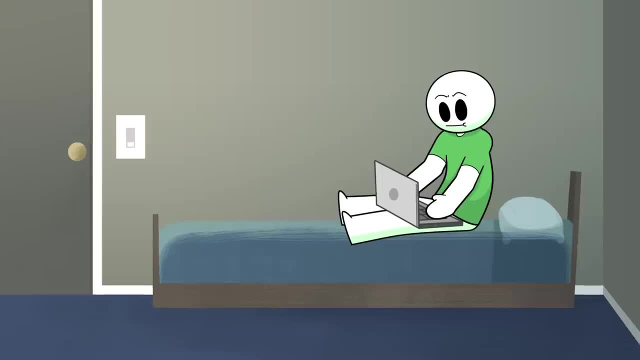 guy casually holding knife. written in my notes- Which, by the way, is actually something I wrote down recently, I don't even- does he just stand there With a knife? Be careful, sir. But this was one of those lucky few times that what I wrote down was actually good. 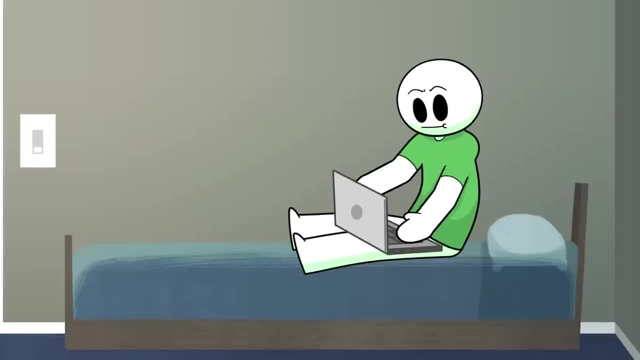 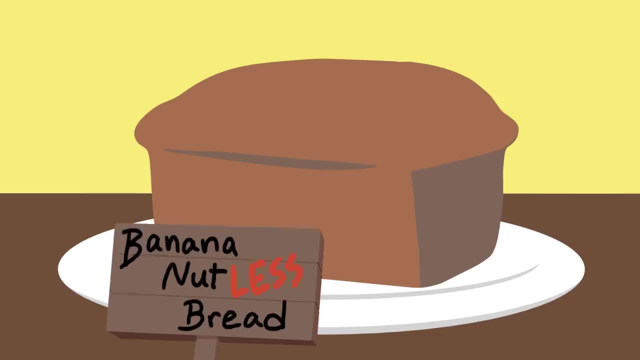 I didn't focus too much on traditions, exactly just a lot of the things I liked about my family, Like how lots of people might make banana nut bread, but since we weren't huge fans of walnuts, we called ours banana nutless bread. I wasn't totally sure what to put on my poster, so I downloaded. 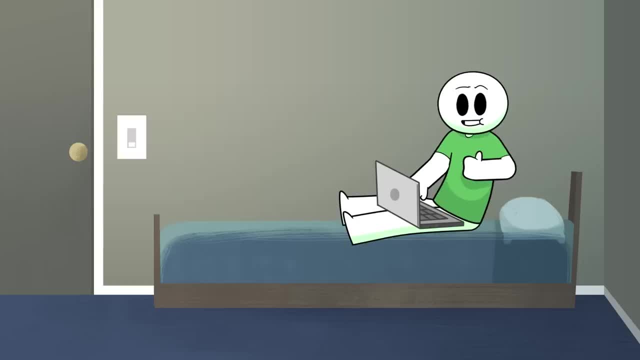 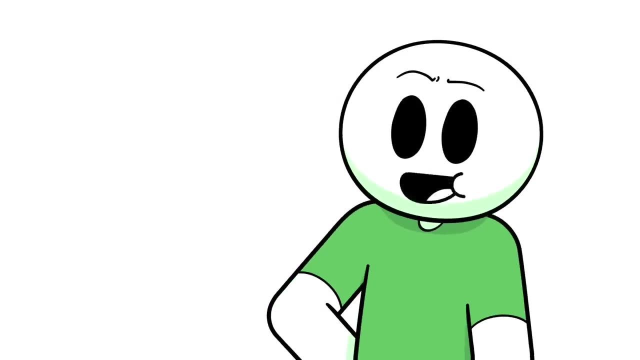 random images of things vaguely related to the stories I was telling, Like a banana And a crab. In the morning I printed off the pictures and frantically glued everything down. Things had turned around completely. I was freaking out just as much, but now it was like a good freak out. 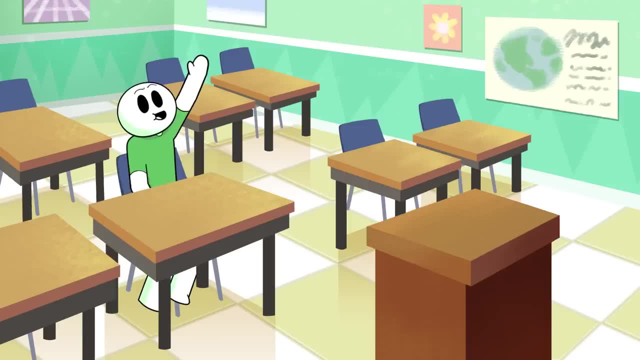 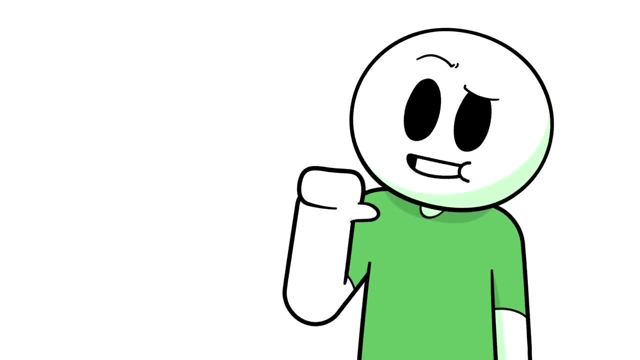 Now that I was prepared. I was actually kind of excited, and during English I volunteered to go first. Everything was fresh in my mind, so I thought I might as well get it out of the way and maybe I could put this good freak out to use. 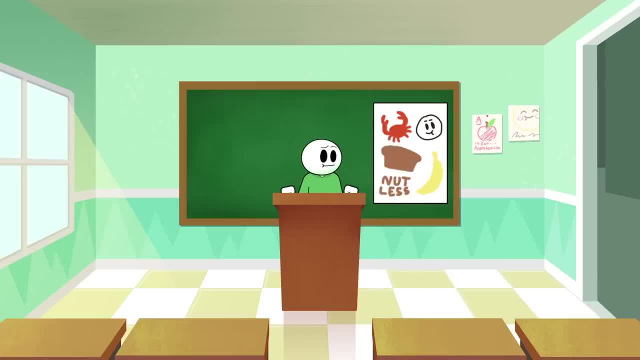 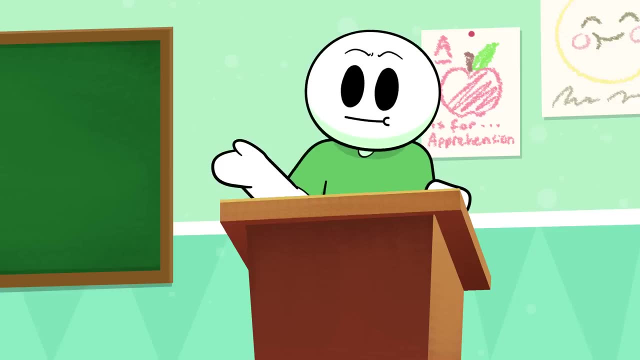 I walked to the front of the room and everyone laughed at how random my poster was. It's always nerve-wracking to give a speech, but banana nutless got a genuine laugh, so that helped. Then I talked about how my grandma had a houseboat, and some of my earliest memories were: 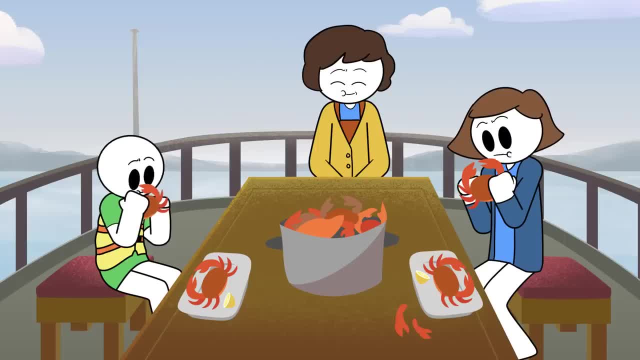 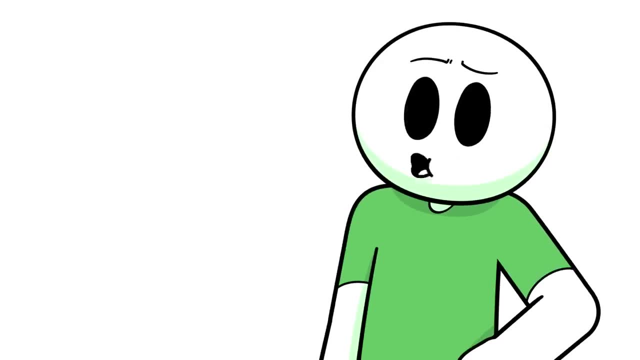 going out on the water to set crab traps. We'd cook the crab right there on the boat and throw the shells back into the water as we ate them, Which sounds super cool, until I tell you Toddler Tim's favorite part of the houseboat Playing McDonald's. That's a game where you run around the. 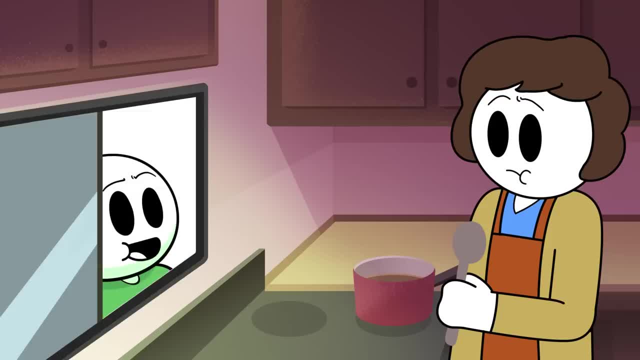 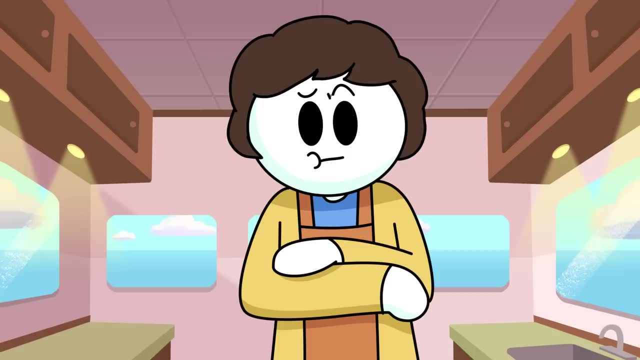 outside of the boat to the kitchen window and knock frantically until your grandma opens up. Then you place your order and run as fast as you can to the window on the other side of the boat to pick up your imaginary food. Rinse and repeat. You'll know you've won when the first window stops. 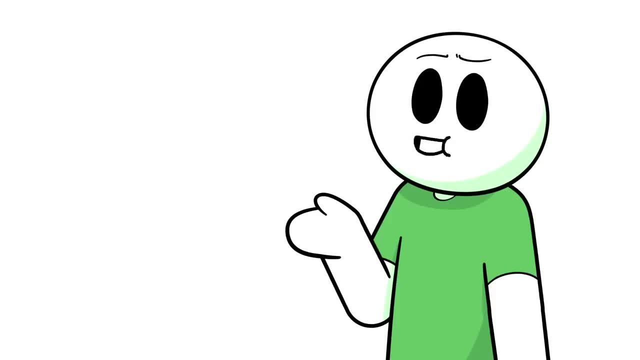 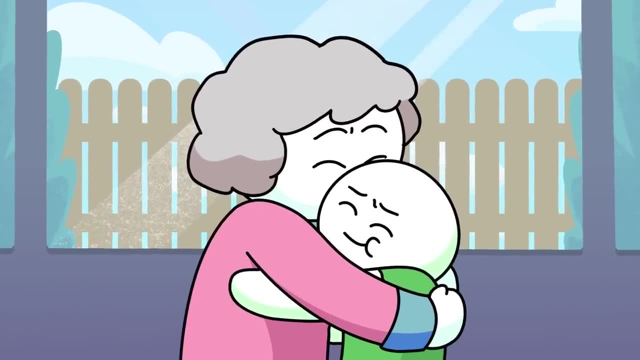 opening, I also talked about my other grandma, Emma. At first she was only my babysitter, but she babysat me from day one and I just grew up calling her grandma. I have so many fond memories of her and when I'm ready I'm going to make a video just for her. 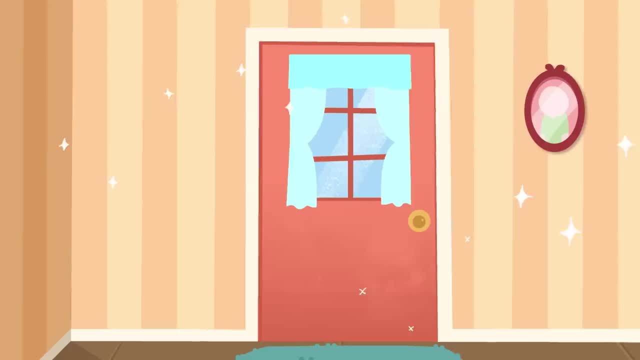 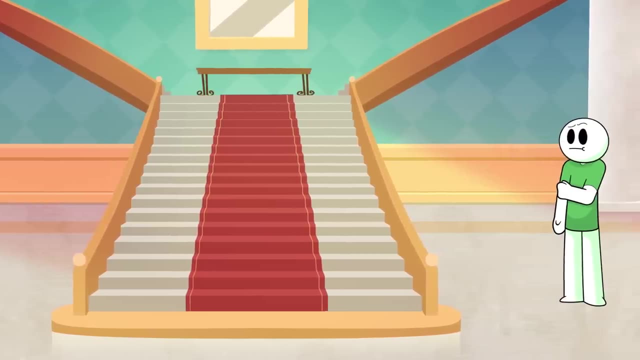 But in the meantime, I'll tell you one of the stories that I shared with my class. Grandma Emma's house was incredibly clean, But you know how some people's houses feel: like a museum, Like they're really clean but also uncomfortable and it's like you're not supposed to touch anything. 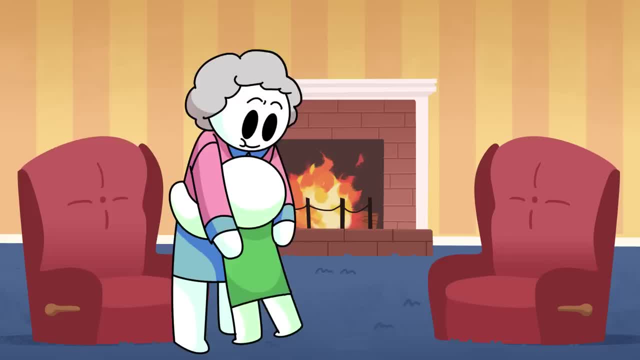 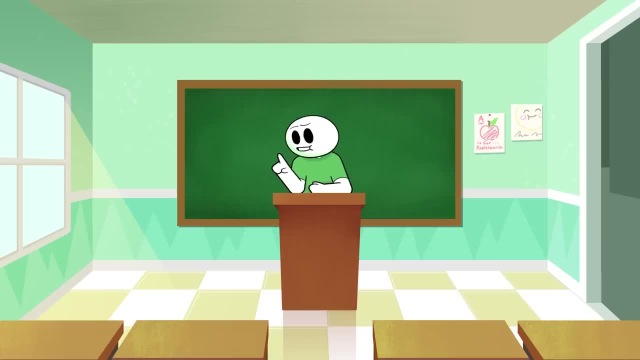 Her house was different. I don't know if it was the lemony fresh smell or her big old grandma hugs, but when you walked in you were home. I told the class that if there's one thing my grandma taught me, it's that you don't have to be blood relatives to be family. Traditions and the 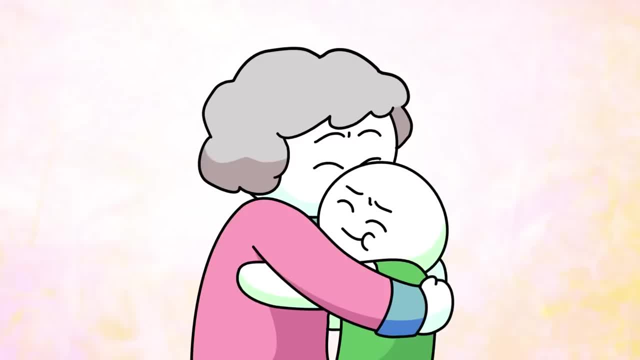 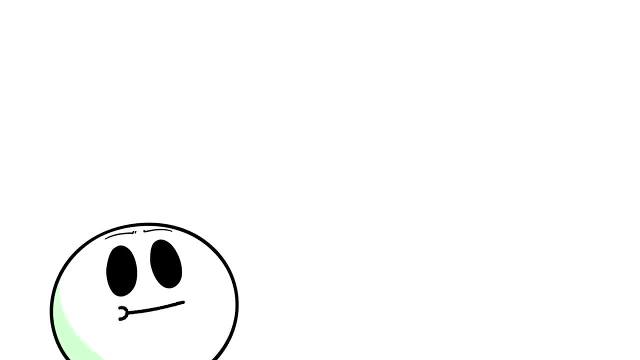 countries they might have come from don't matter In the end. the only thing that matters are the memories we have of the ones we love, Or something like that. Maybe the universe is a hologram and nothing matters. The point is the class freaking loved my speech. I'd like to think it. 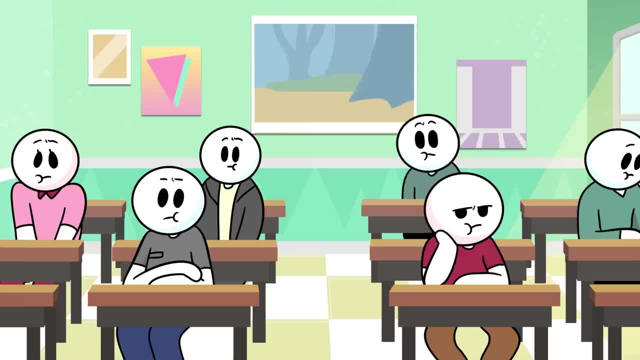 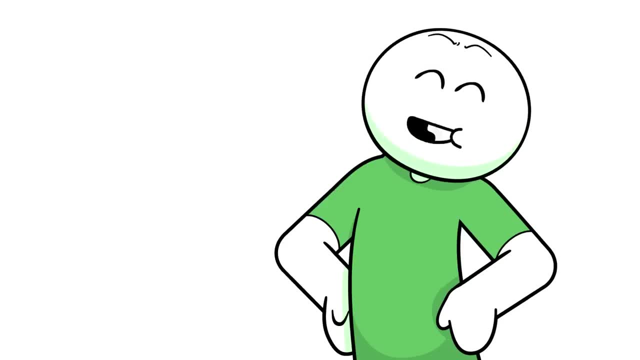 was because I shared something really personal, but it was probably because I ended by essentially saying that this whole assignment was worthless and everyone was like, yeah, stick it to the man. Whatever the reason, I got an honest-to-goodness standing ovation. Now I don't blame those of you. 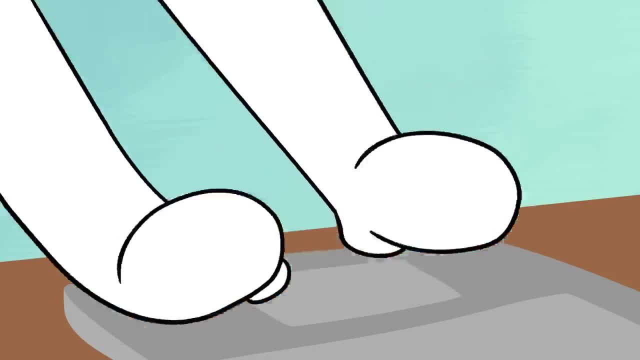 in the comments with your little jazz hands saying that there's no way I got a standing ovation at school. but I don't care what you think, because I know the truth and that's all that matters, Unless we're holograms. 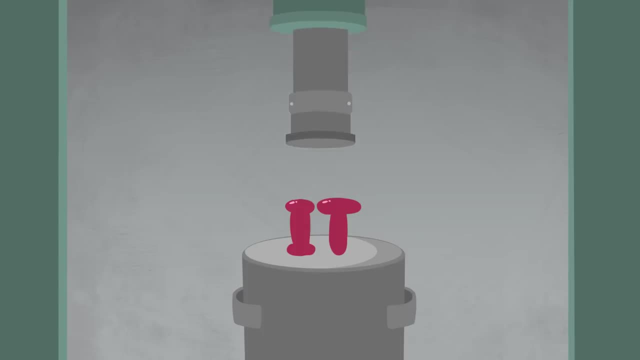 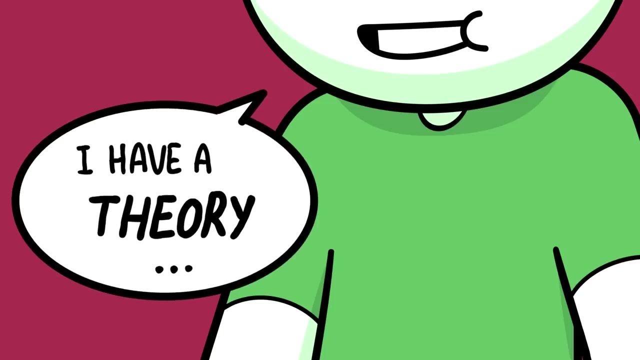 Anyway, I love giving presentations. I think I had to totally crush it at least once to realize how it can be. but now I love performing. I still get nervous, but here's my secret to dealing with it. I have a theory, A regular theory. 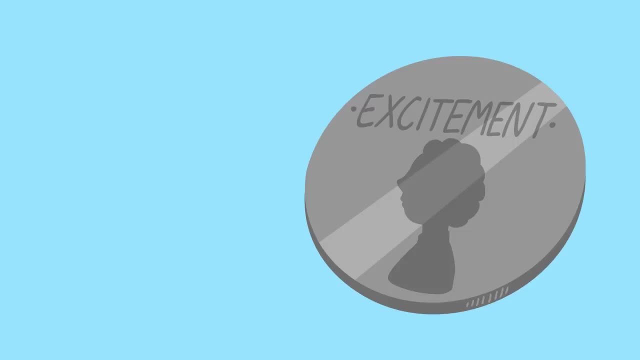 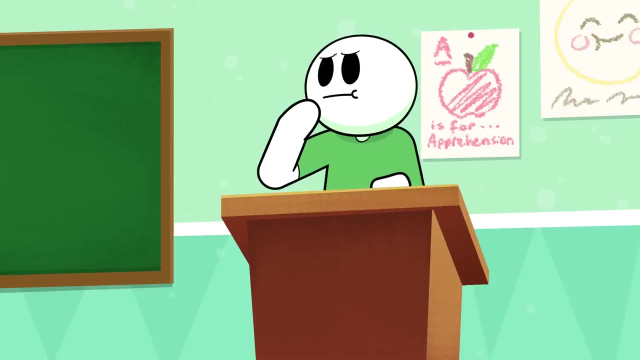 Giving a speech is an intense experience, but I think anxiety and excitement are kind of two sides on the same intensity coin, if that makes sense. When you're about to perform, you get a hit of adrenaline and most people feel that as anxiety. But I've found that most 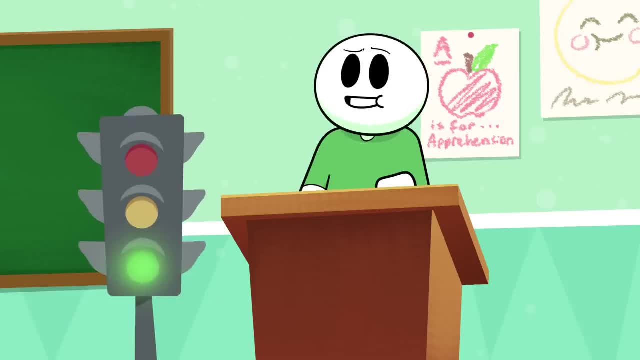 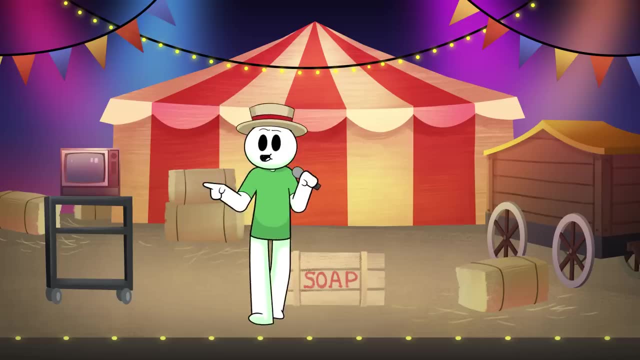 of the time, I can decide to feel that intensity as excitement instead, Especially if I've prepared and know exactly what I'm supposed to say. It doesn't work every time, but it's worth a shot. So the next time you give a presentation, try your best not to feel hesitation. Remember to 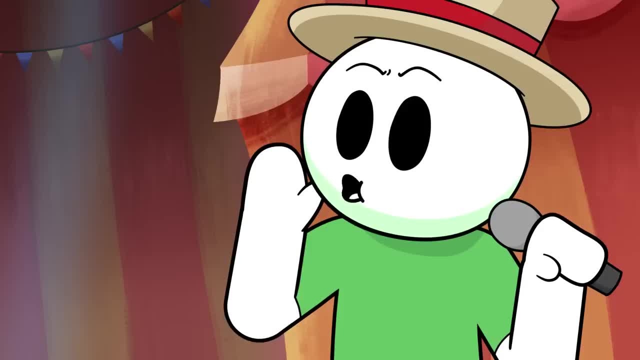 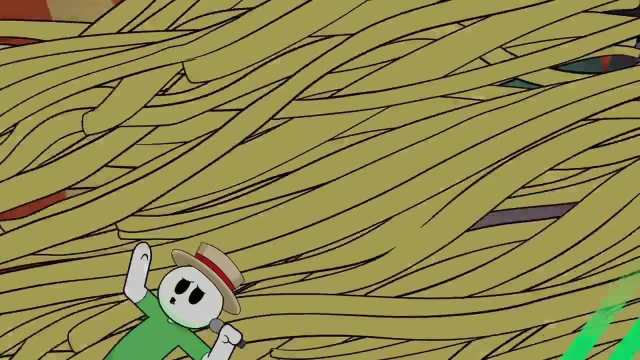 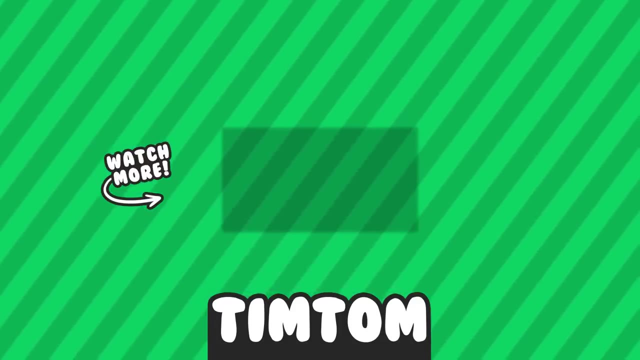 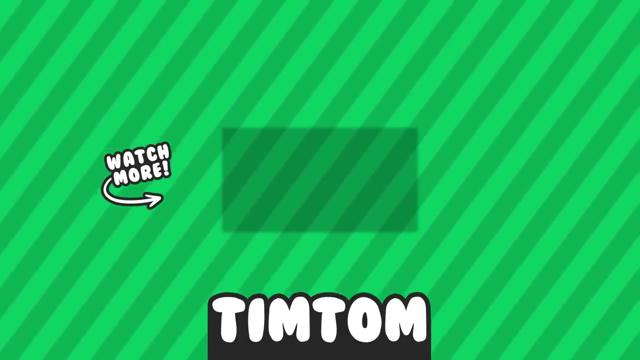 turn your fear into fuel. Classmates will stand and shout that you ruled And after you'll say, oh, no way it is possible. I never should have left that comment on Tim's video. I hope you enjoyed this video and I'll see you in the next one.